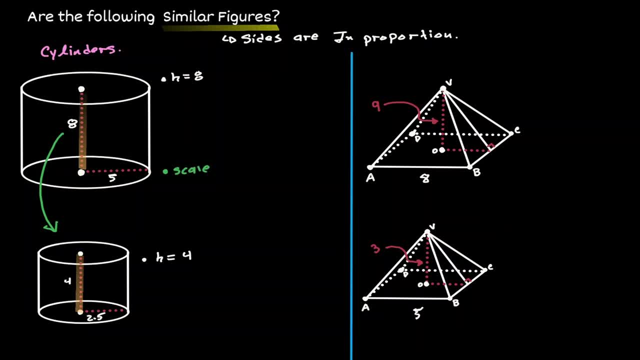 and end up with the cylinder on the bottom. we can define the scale factor by obtaining the height of one figure and divided by the height of the other figure. We are comparing the same characteristics between two figures, so we will have four over eight. 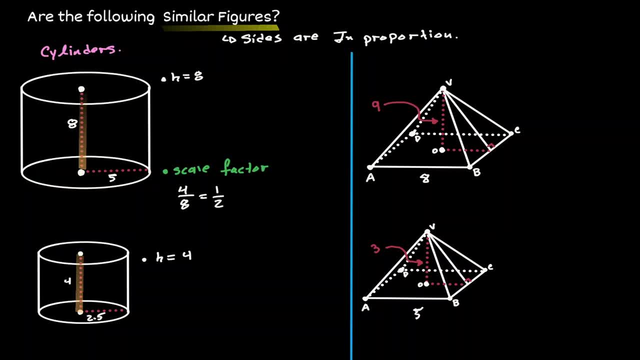 which is equivalent to one half, Just by comparing both heights. it's not sufficient to define the scale factor. We have to confirm it. Well, let's see if we obtain the same value when we compare the radius of the upper cylinder with the radius of the lower cylinder. 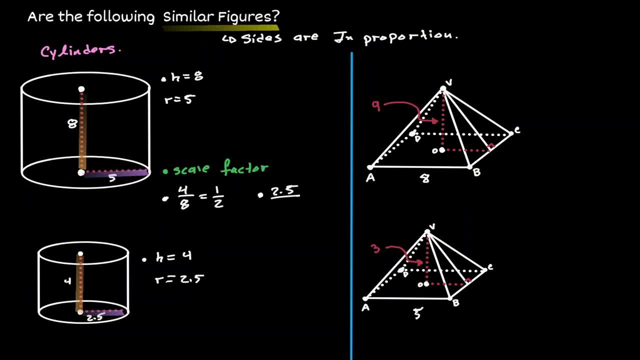 Let's see what we get. when we divide 2.5 over five, We are comparing both radiuses, And when we do notice that this is also one half, When we compare both height of this cylinder, we obtain a ratio of one half. 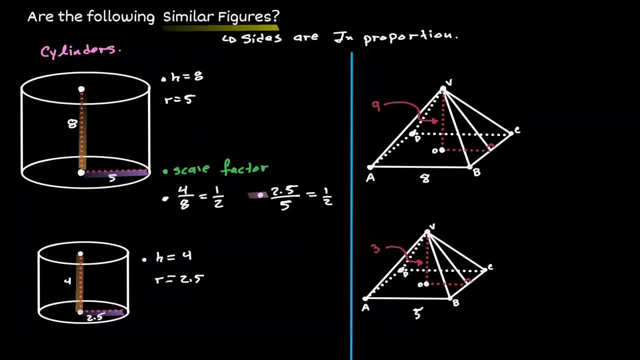 And when we compare both radiuses of the cylinders we also got one half. Then we can determine that the sides of these figures are in proportion and we can conclude that we have similar figures with the scale factor of one half. Now let's concentrate on the two pyramids. 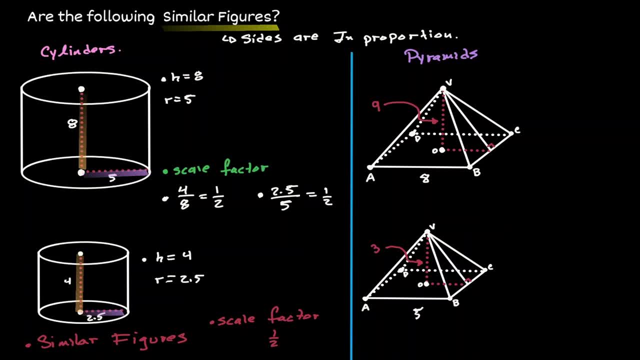 on the right-hand side. Let's try to determine if both pyramids have a scale factor. Let's start by comparing the height of the pyramid on top with the height of the pyramid on the bottom. The height is nine on top and the height is three on the bottom. 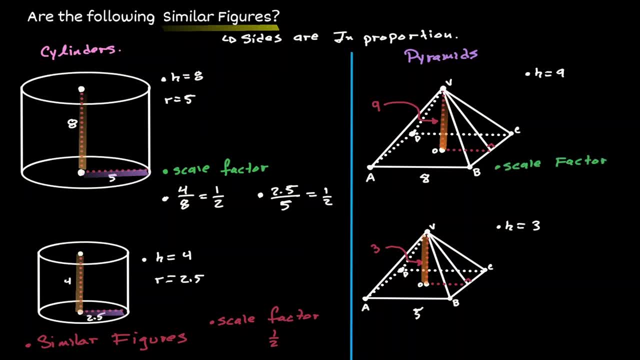 So one possible scale factor will be of three divided by nine, which is equivalent to one third. Now let's just compare another sides of these two pyramids and see if we also get one third when we're looking for a proportion. Notice that on the pyramid on the top. 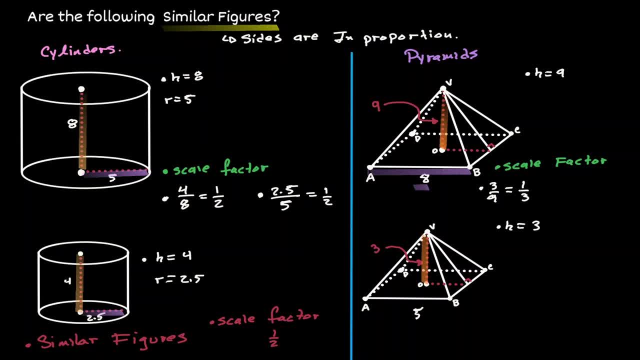 one side of the base is of a value of eight and the same side in the other pyramid it holds a value of five. Let me move this information a little bit to the bottom. Notice that when we compare those two sides, if we get five and we divide it by eight, 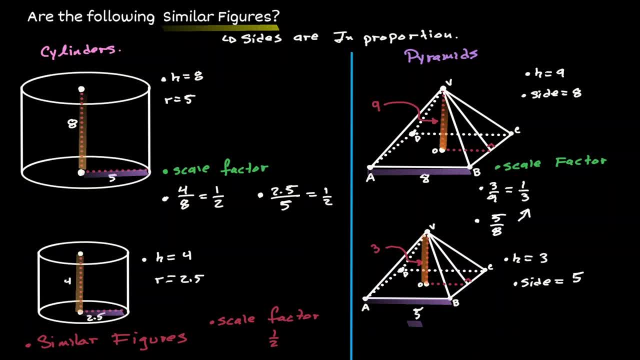 that is not equivalent to the scale factor that we got when we were comparing the height of those pyramids. because these two values do not match up, then we will conclude that these two pyramids are not in proportion. Therefore, these two figures are not similar figures. 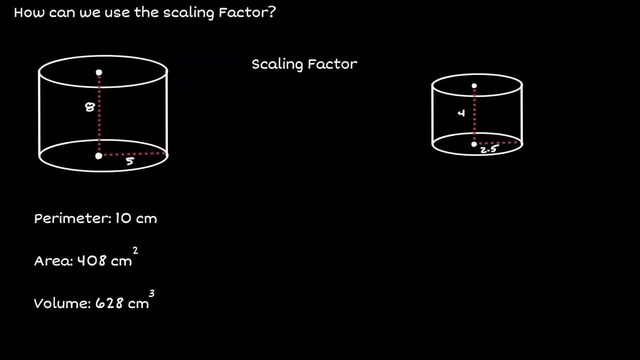 Now let's discuss one application: the scale factor. So here we have two cylinders which we already shown that they are similar figures And in addition we have shown that when we compare the height of both cylinders and when we compare the radius of both cylinders, 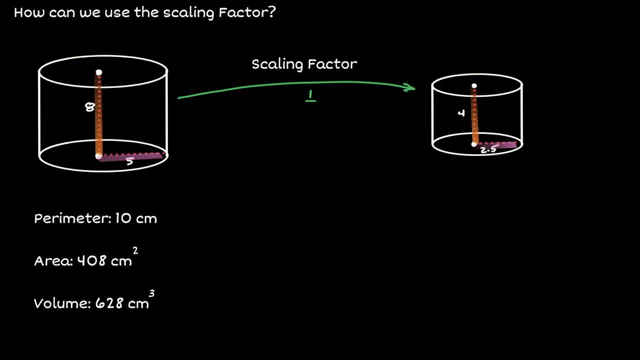 we obtain the scale factor of a value of one half. One way to make sense. notice that eight. if we multiply by one half, we obtain four, and five. if we multiply by one half, we obtain 2.5.. And now let's say that we have more information. 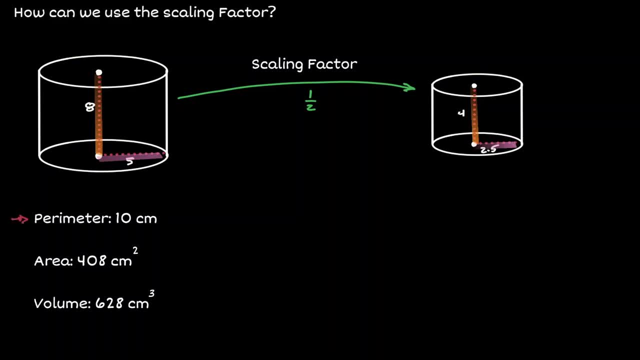 on the cylinder on the left. We know that the perimeter of this cylinder has a value of 10 centimeters And just knowing the scale factor can we define the perimeter on the cylinder on the right? And we can, because if we obtain the perimeter, 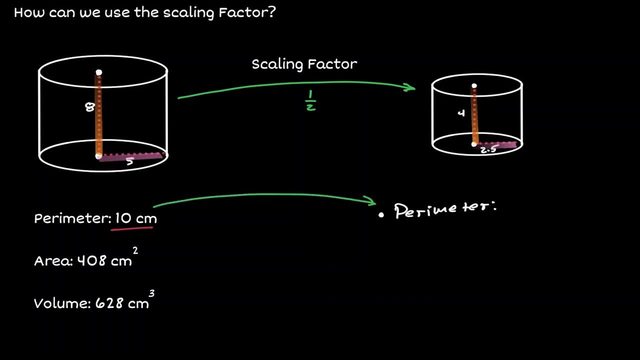 on the cylinder on the left and we multiply by the scale factor, which is one half, that is going to give us the perimeter of the similar figure which is the cylinder on the right. But if we get 10, and we multiply it times one half, 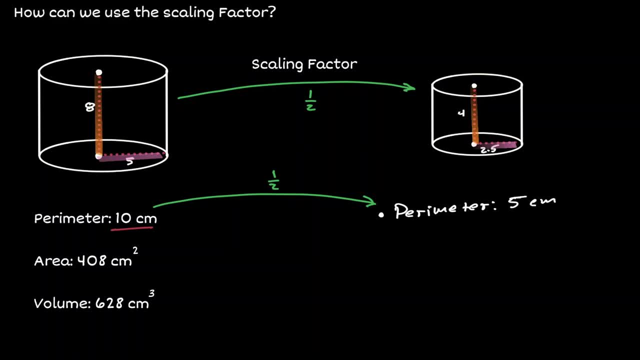 we will obtain five centimeters. If two figures are similar and they have a scale factor, then we can obtain the perimeter of one figure, multiply it times the scale factor and obtain the perimeter of the second figure. But how about the area? 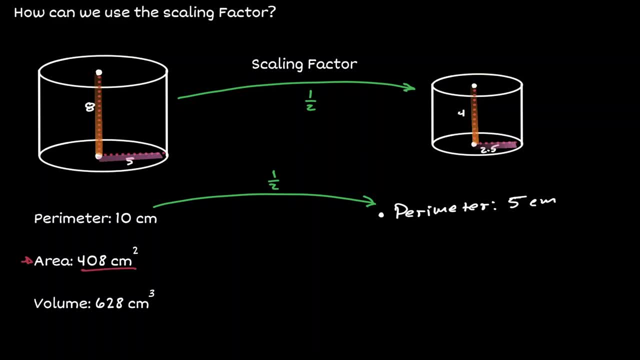 Let's say that we know that the area on the cylinder on the left will be of 408 centimeters squared. Do we have enough information to find the area of the cylinder on the right? We can use the scale factor, but now we're not going to multiply times one half. 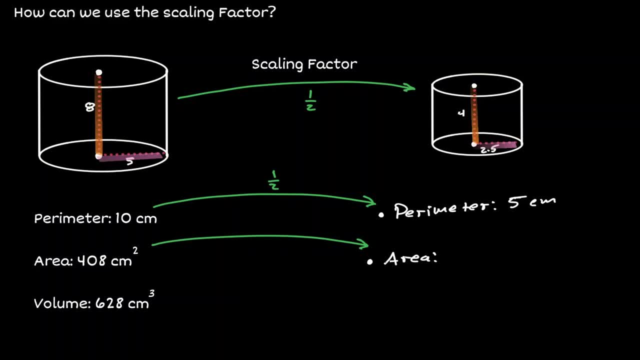 Notice that the units of areas are always given in square. so to obtain the area of a similar figure, we will get the scale factor where. So, if we get 408,, which is the area on the figure on the left, and we multiply it times one half,